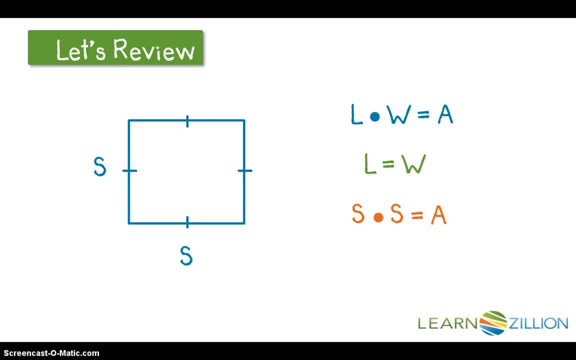 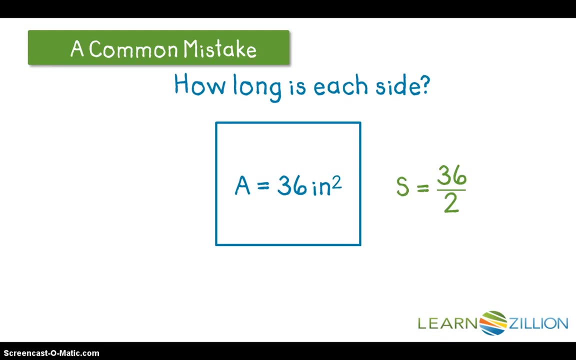 So to find the area, you simply multiply one side length by itself. Multiplying a number by itself can also be expressed as raising that number to the second power. Here's a common mistake. Sometimes, when students see a question like this, they decide to divide 36 by 2.. 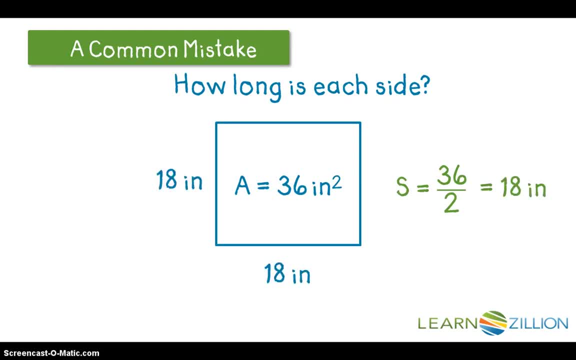 But 36 divided by 2 is 18.. If the side length were 18, to find the area we'd multiply 18 times 18.. That results in 324 inches squared, not 36.. So dividing by 2 is not the way to find the side length. Others may divide the side length by 4, because they see 4 sides. 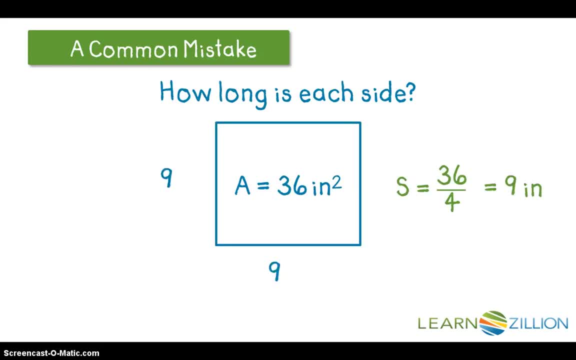 But 36 divided by 4 is 9.. If the side length of the square were 9, the perimeter would be 36, because that's 9 plus 9 plus 9 plus 9, but the area would be 9 times 9.. 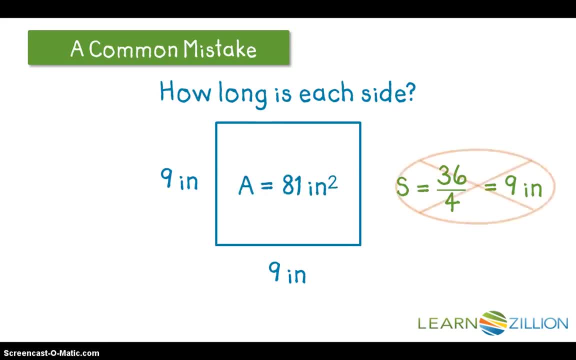 Which is 81, not 36.. So we also do not divide the area by 4 to find the side length. So we don't divide by 2, we don't divide by 4.. What should we do? Since this square has an area of 36, and since we find the area by multiplying the side length by itself? 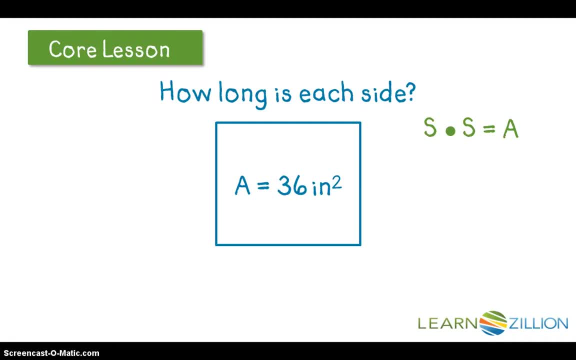 the side length of this square has to multiply by itself to equal 36.. Can you think of a number that multiplies by itself to give us 36?? It turns out that number is 6.. 6 times itself is 36.. So a square that has a side length of 6 would have an area of 36.. 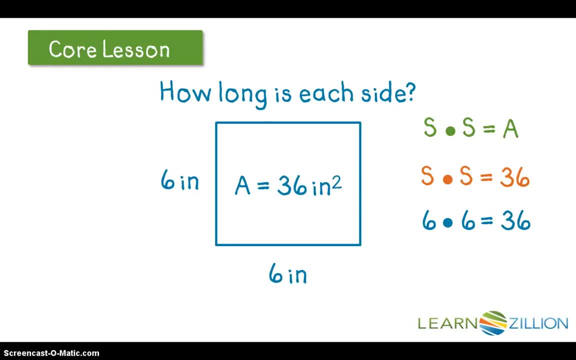 This is the side length we were looking for. This square is 6 units long by 6 units wide, Because we will always find the area of a square by multiplying a number by itself and because multiplying a number by itself can be represented by using an exponent of 2,. 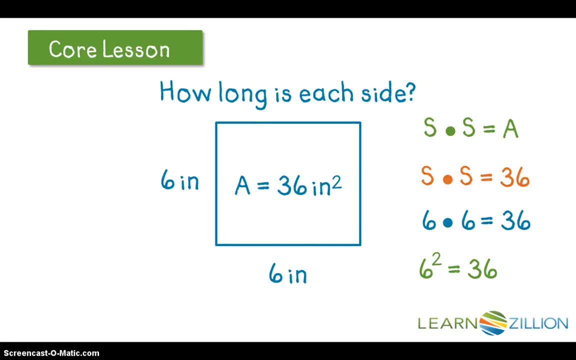 raising a number to an exponent of 2 is often called squaring a number. So we can say this is 6 to the second power, or we can say 6 squared. To review this process, when we wanted to find the side length of a square that had an area of 36,, 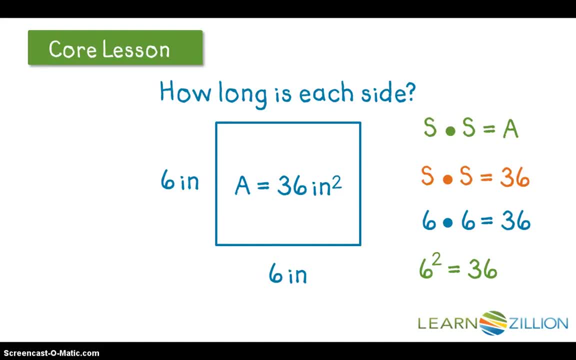 we needed to find a number that, when multiplied by itself, gave us 36.. That number turned out to be 6 inches. Here's another example. This time we are trying to find the side length of a square that has an area of 80 centimeters squared. 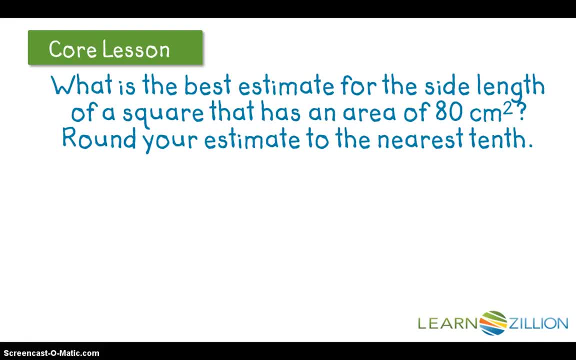 But it's asking us to estimate our answer to the nearest tenth. I wonder why We know we're supposed to square the side length to get the area, but squaring a side length means we're supposed to multiply the side length by itself. 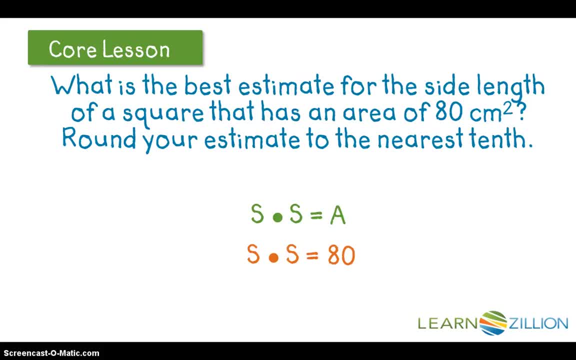 This specifically means in this problem we're supposed to multiply the side length by itself and get 80. I know that if the square has a side length of 8, the area would be 8 squared, which is 8 times 8, which equals 64.. 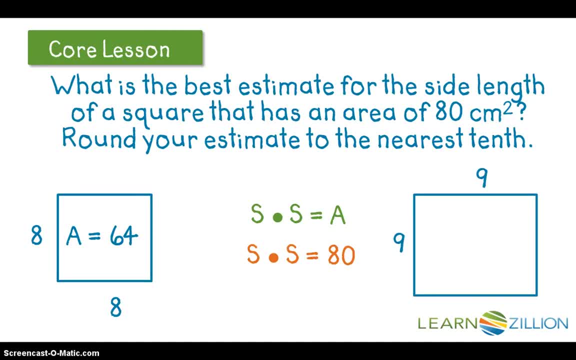 That's too small. But if the side length were 9, we'd find the area by multiplying 9 by itself, which is 81. That's too big. Let's go ahead and move to a clean page so we can get some space here. 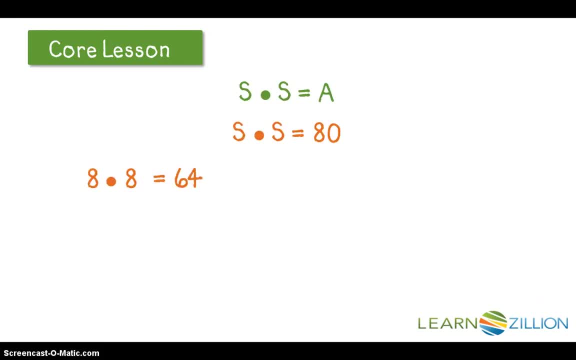 So if our side length were 8,, the area of the square would be 64.. That's too small, so that means our side length must be bigger than 8.. But if our side length were 9,, the area would be 81.. 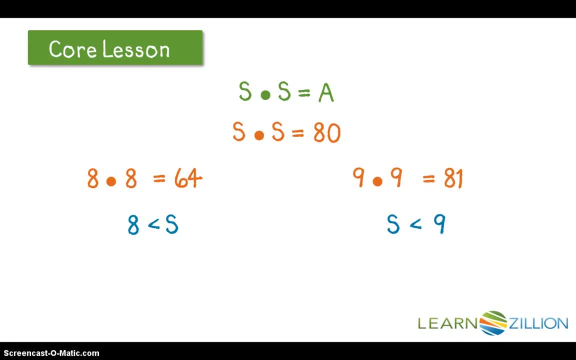 That's too big. so our side length must be smaller than 9.. Our side length has to be bigger than 8, but smaller than 9.. But where, Well, 80 is just a little bit smaller than 81. So perhaps our side length should be just a little bit smaller than 9.. 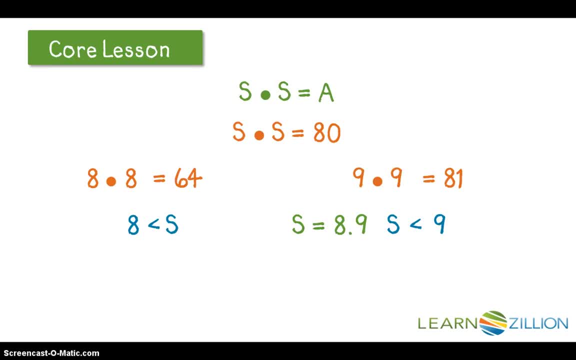 Let's try 1 tenth smaller, or 8.9.. If 8.9 were our side length, we would find our area by multiplying 8.9 by 8.9.. That equals 79.24.. This is not exactly 80,, but it's less than 1 away. 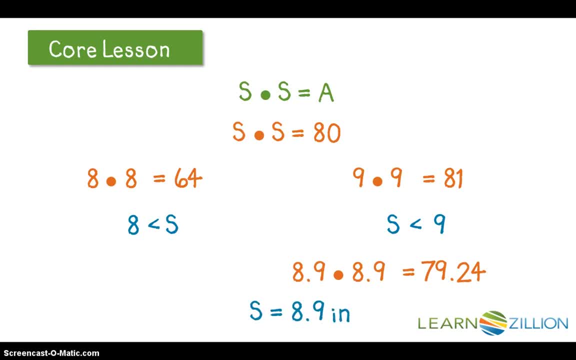 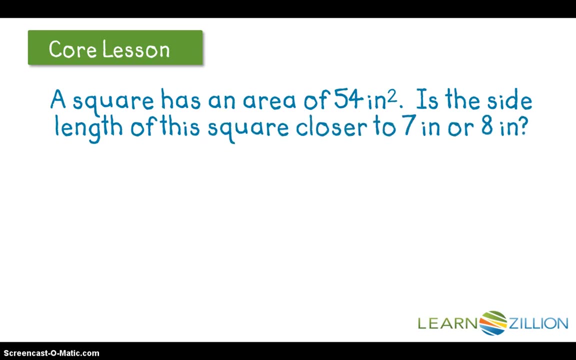 which is a closer estimate than 81 was. So we'll go ahead and estimate the side length of this square as 8.9 centimeters. This last one is asking us to determine whether the side length of a square that has an area of 54 inches squared would be closer to 7 inches or 8 inches. 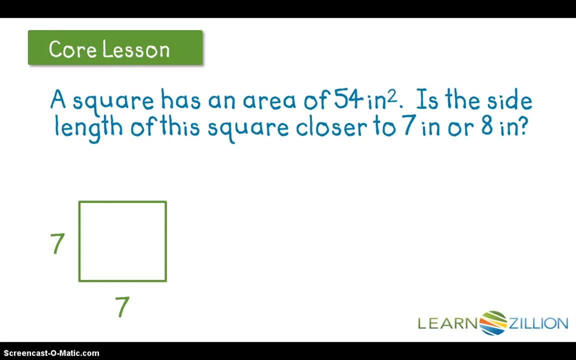 Let's check each side length first. A side length of 7 would have an area of 49. A side length of 8 would have an area of 8 times 8, or 64. So the area of 54 comes from a side length that's got to be somewhere in between 7 and 8.. 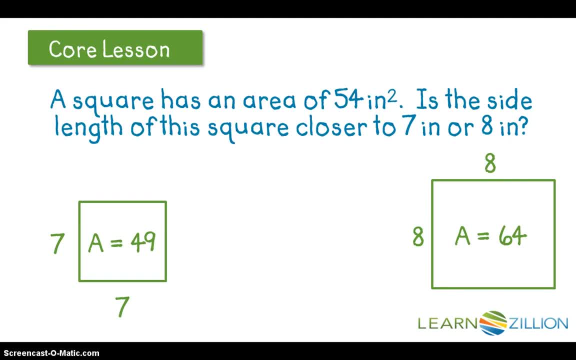 An area of 54 is 10 away from 64, but it's only 5 away from 49. Since 54 is closer to 49, its side length would be closer to 7.. We can answer this question by saying that the side length would be closer to 7 inches.